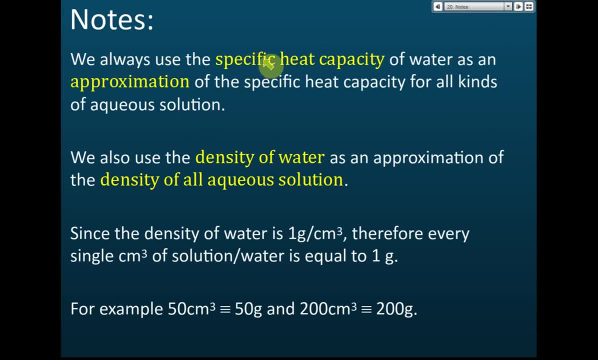 we need to know first. we always use the specific heat capacities of water as an approximations of the specific capacities of all kinds of aqueous solutions in chemical reactions. the solutions that we use that may be like acid or alkali or salt. maybe the solution is sodium hydroxide. okay. 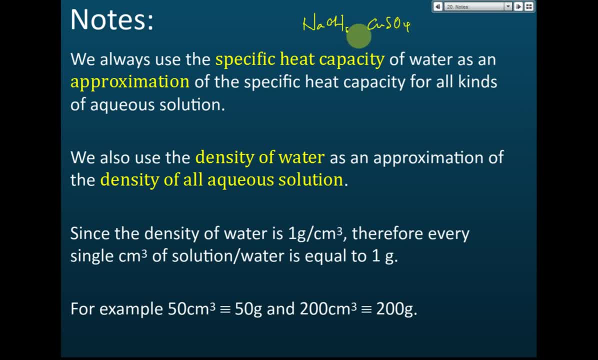 or maybe it's a copper sulfate solution. all this is aqueous solutions, aqueous solutions. now. for aqueous solutions, the specific heat capacity will be slightly lower than the specific heat capacities of water. for example, the specific heat capacities of water is 4200, so for sodium hydroxide maybe is 4150 only, or maybe for copper sulfate is 4125. okay, 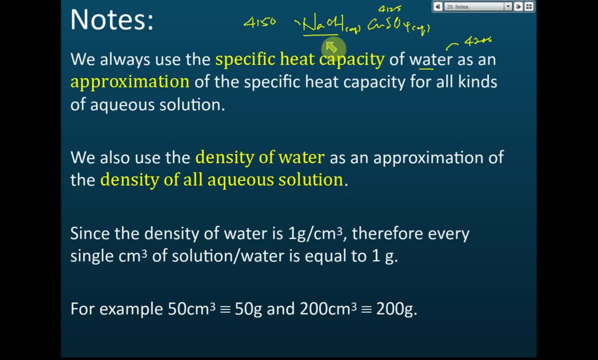 the specific heat capacities of the aqueous solution may be slightly lower than the specific heat capacities of water, but in spm. in spm we always use the specific heat capacities of water as the approximations to the specific capacities of the equal solutions. so no matter is sodium hydroxide or copper. 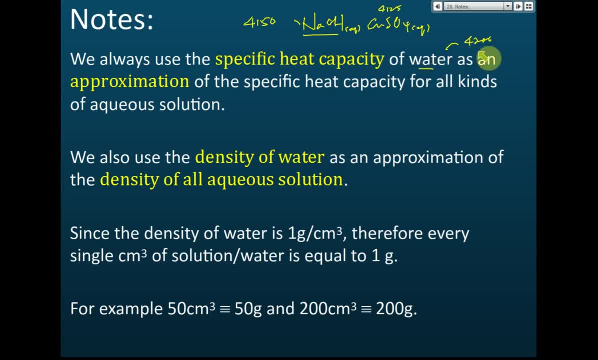 sulfate. we assume that the specific heat capacity is the same as the specific capacities of water, so you don't need to worry about the solutions because some students say, oh, this is copper south, it's not water. so can we use uh, specific heat capacities of water for the calculation? 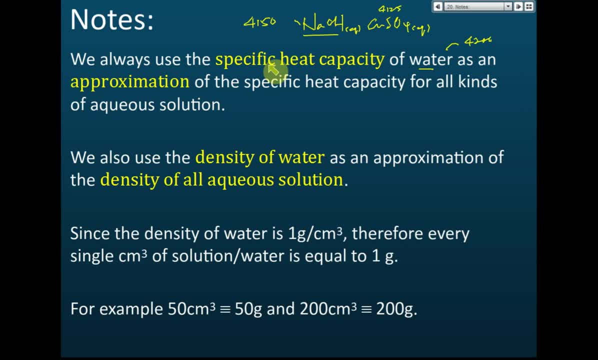 Yes, you can use the specific heat capacities of water for the calculation, because it's very close. The specific capacities of the aqueous solution is very close to the specific specific heat capacities of water. So that is the first things that you need to know. 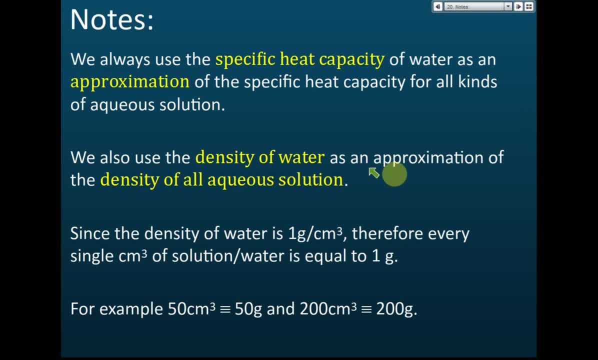 The second one is: we also use the densities of water as an approximations of the densities of all aqueous solutions. The densities of water is one gram per cm cube. OK, one gram per cm cube, But for aqueous solutions the density will be higher. 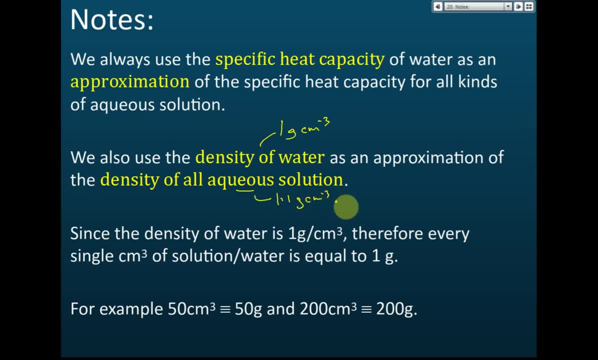 Maybe it's one point, one gram per cm cube or something like this. OK, so the density is slightly higher, But, but no matter what's the densities of the solutions. we always use the densities of water as the approximations to the densities of all aqueous solutions.